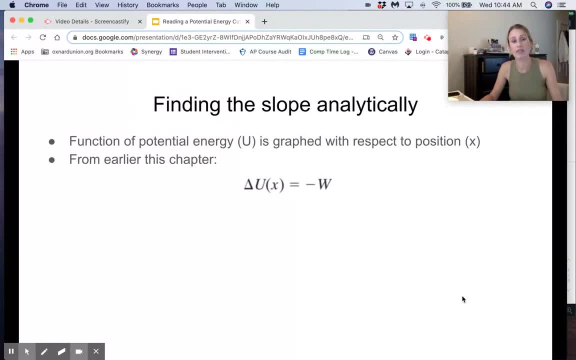 potential energy as a function of position is equal to the negative work done on the object. So if we remember that work is equal to force times, displacement times, the cosine of theta, we get that the change in potential energy is equal to negative force with. and then 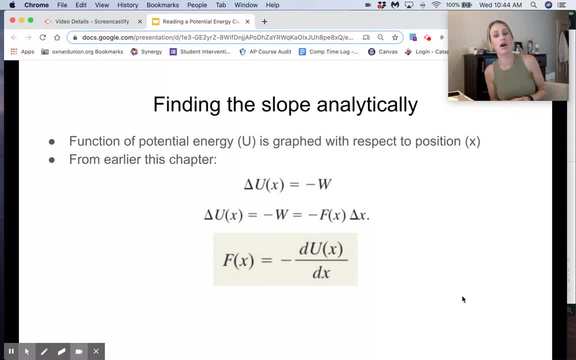 multiplied by the force, by displacement. So here, if we solve this equation for force, what we get is the change in potential energy over displacement. So here, what this tells us is that when we look at the slope here, which is just going to be change in potential energy over displacement, or delta u. 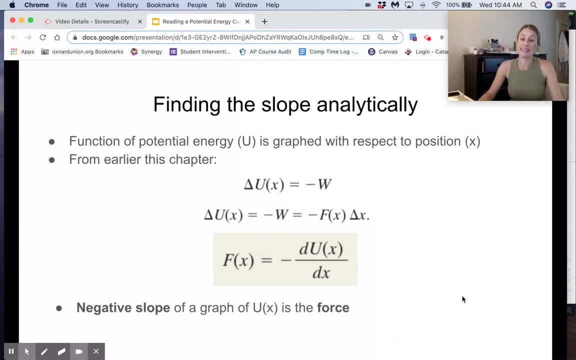 over delta x, we are going to get a negative force. If you multiply both sides of this equation by negative one, you get du over dx equals negative force. So the negative slope of the graph is going to be the force, and this is really really important to remember here. Also, if we take the 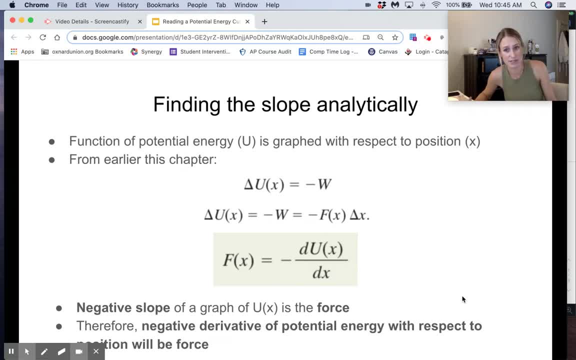 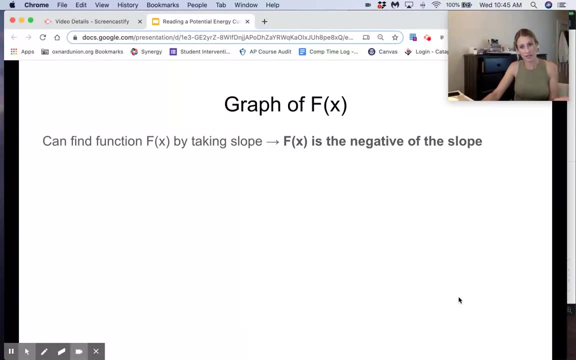 derivative of the potential energy function with respect to position, we get the negative force as well. So you take the derivative, slap a negative on there and you then get your force. So if we graph the force, then from the potential energy graph it's going to look something like this: So again, 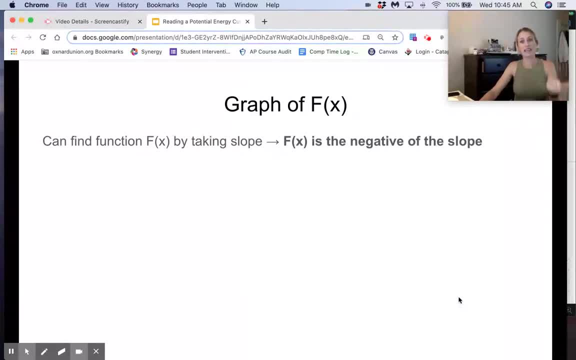 when we're looking at that force, it's the negative of the slope. So if I have something like this, our potential energy graph with respect to position, here we want to look at what's happening to slope, So at this position, or sorry, this part of the graph right here. so until about. 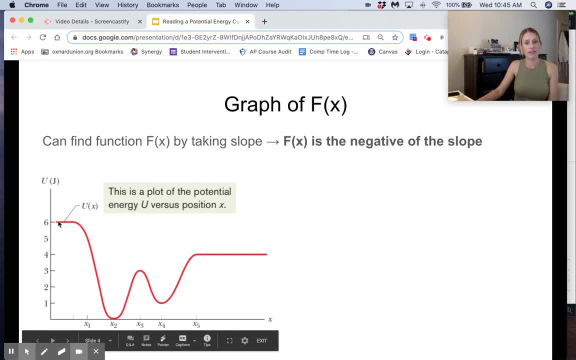 x equals x1, we have no slope, So we start at a force of zero. Then we start with a negative slope, which means that we have a positive force. Negative slope means positive force, because the slope is the negative force. Now down here, at x equals two, again we have a slope of zero. So that means we have no force. 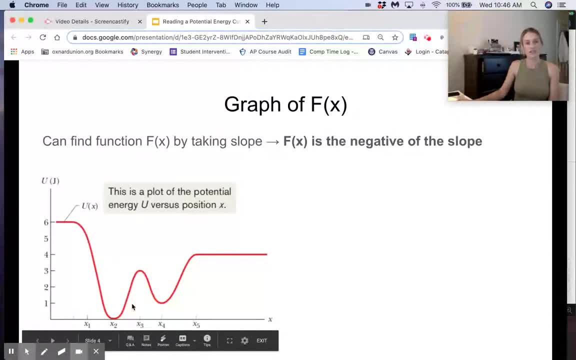 at x equals two, And then we start getting a positive slope which tells us that we have a negative force At x3, we again we have a negative force, So we start at a negative force Again, have a slope of zero, So we have no force at x3 or at x4.. We can see that, But between x3 and 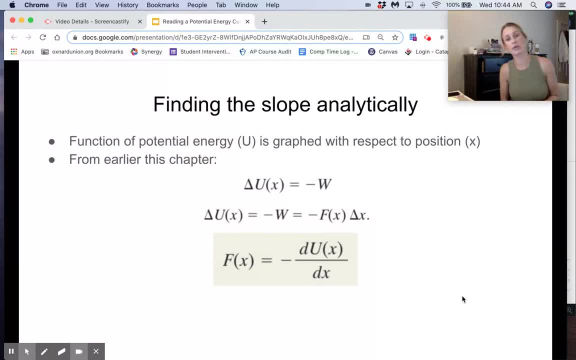 by the force of the force, And so we get that the force of the object is equal to negative force by displacement. So here, if we solve this equation for force, what we get is the change in potential energy over displacement. So here, what this tells us is that when we look at the 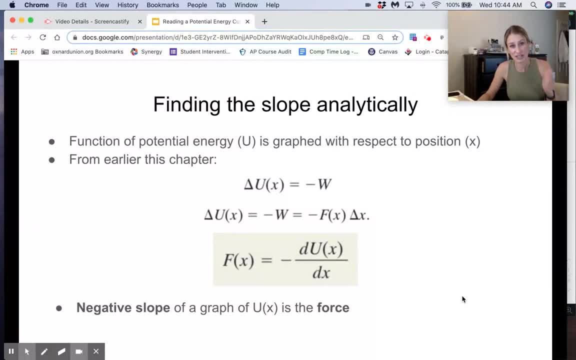 slope here, which is just going to be change in potential energy over displacement, or delta u over delta x, we are going to get a negative force. If you multiply both sides of this equation by negative one, you get du over dx equals negative force. So the negative slope of the graph is going. 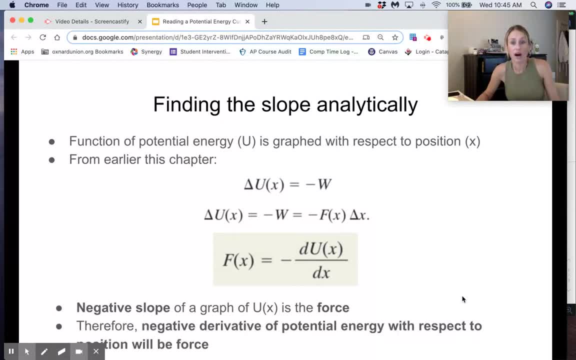 to be the force, and this is really, really important to remember here. Also, if we take the derivative of the potential energy function with respect to position, we get the negative force as well. So you take the derivative, slap a negative on there and you then get your force. So if we 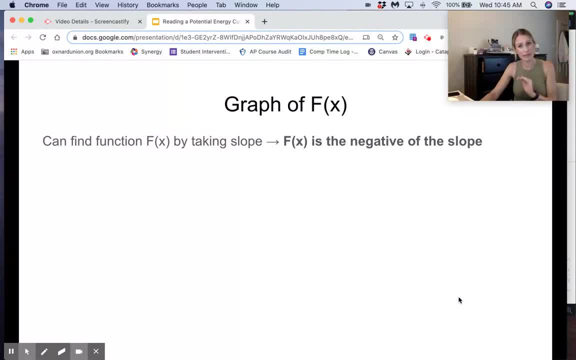 graph the force. then, from the potential energy graph, it's going to look something like this: So again, when we're looking at that force, it's the negative of the slope. So if I have something like this, our potential energy graph with respect to position, here we want to look at what's. 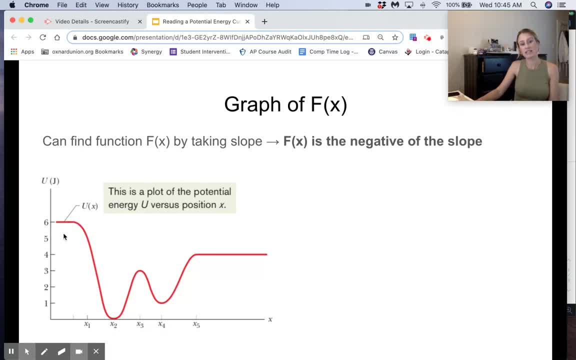 happening to slope. So at this position, or sorry, this part of the graph right here, so until about x equals x1, we have no slope. So we start at a force of zero, Then we start with a negative slope, which means that we have a. 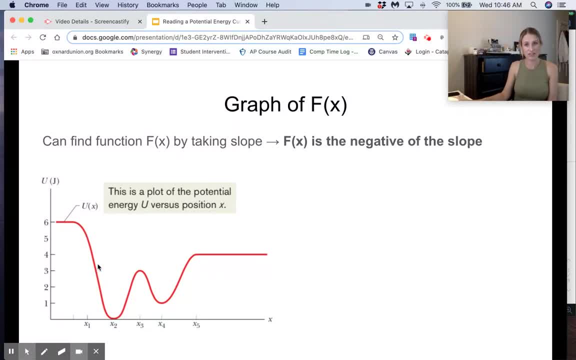 positive force. Negative slope means positive force because the slope is the negative force. Now down here, at x equals two, again we have a slope of zero. So that means we have no force at x equals two. And then we start getting a positive slope which tells us that we have a. 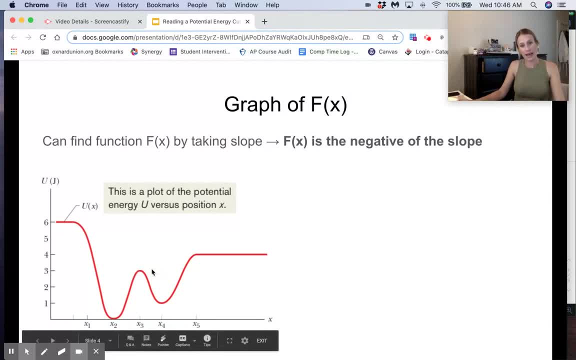 negative force At x3, we again we have a negative force, So we start at a negative force Again, have a slope of zero, So we have no force at x3 or at x4.. We can see that, But between x3 and 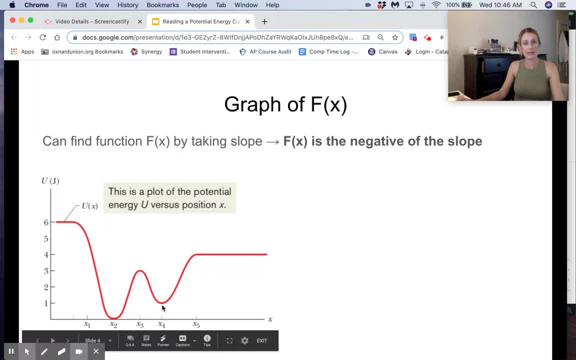 x4,. again we have a negative slope here, which means we have a positive force. And then between x4 and x5, we have a positive slope, which means negative force. So if we look at something like this, again we have no force. So force equals to zero Here where we have a slope of zero. 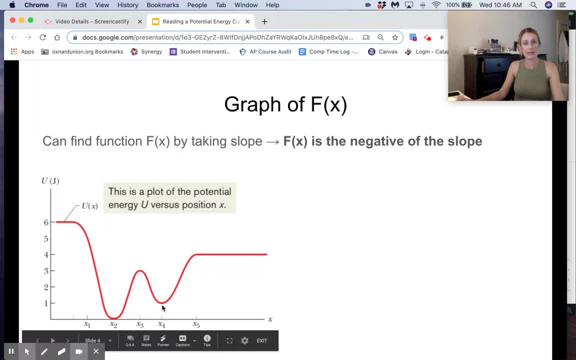 x4,. again we have a negative slope here, which means we have a positive force. And then between x4 and x5, we have a positive slope, which means negative force. So if we look at something like this, again we have no force. So force equals to zero Here where we have a slope of zero. 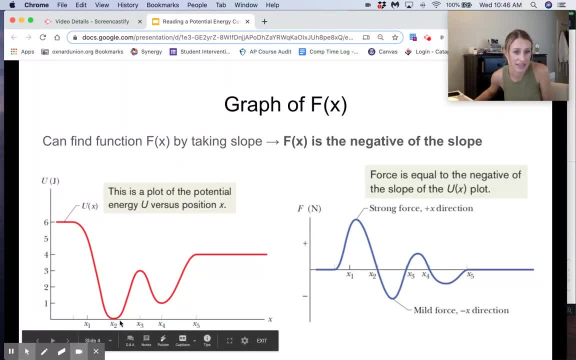 at x equals two. So we can see that We have a slope of zero here At x equals three. slope of zero here At x equals four. slope of zero here, And then after x equals five. slope of zero here, And then, as we go down here, 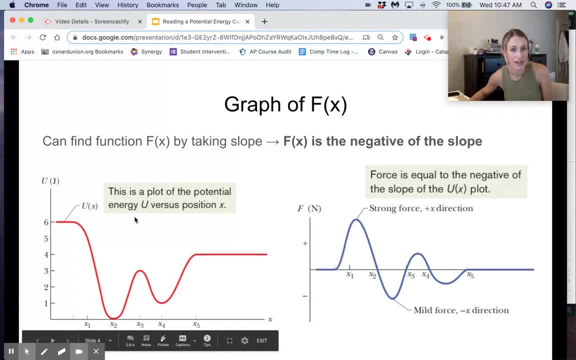 this is a negative slope. We have a positive force right here, And then here we can see that the slope is increasing, which means that the force is increasing. Here we have our largest positive force, And then it's going to decrease back to zero, which is why we're coming back down. 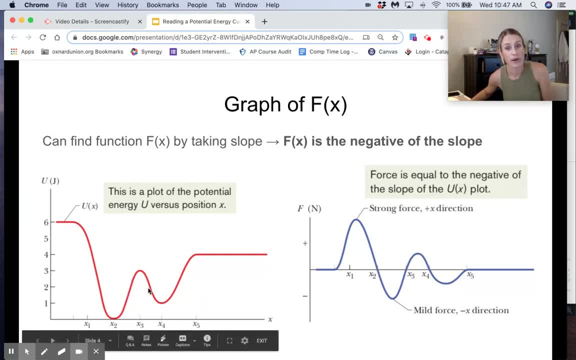 to zero here. Here our slope is lower in magnitude, so it doesn't get as high as here. but because it's a positive slope here, that means it's a negative force. and then here we have a slope that is negative, so we have a positive force here. and then here we have a positive slope, so we have 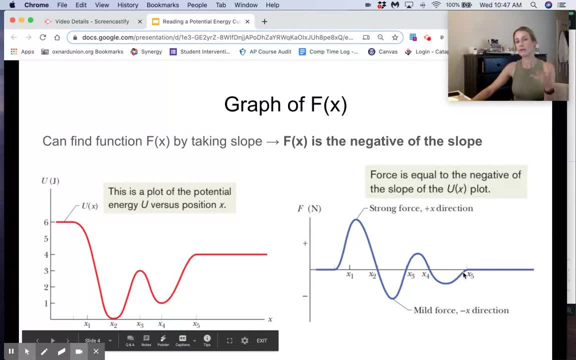 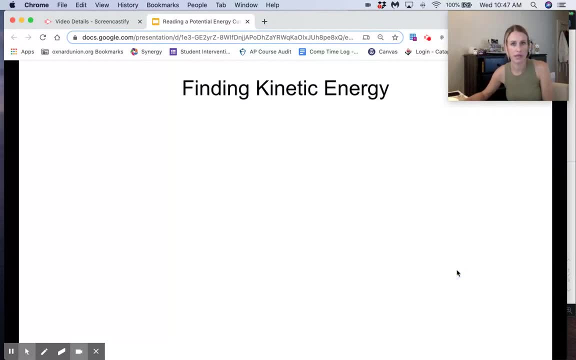 a negative force here. So you can kind of see how we could get a force graph from our potential energy graph. Now if we're trying to find kinetic energy from potential or a potential energy graph, we have to remember that mechanical energy of a system has a constant value that's given by 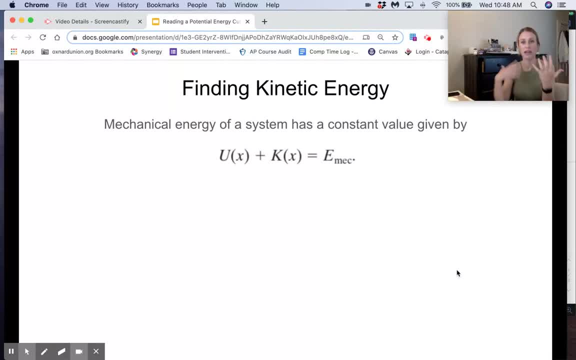 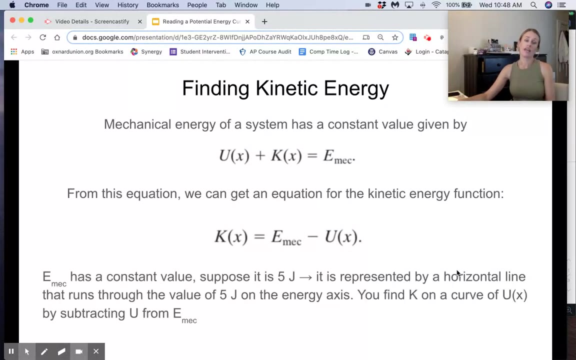 this right here: Mechanical energy is equal to a combination of potential energy plus kinetic energy. So from this equation we can get an equation for the kinetic energy function We get. kinetic energy is equal to total mechanical energy minus potential energy. So if we know that the total mechanical energy has a constant value, which we know from conservation, 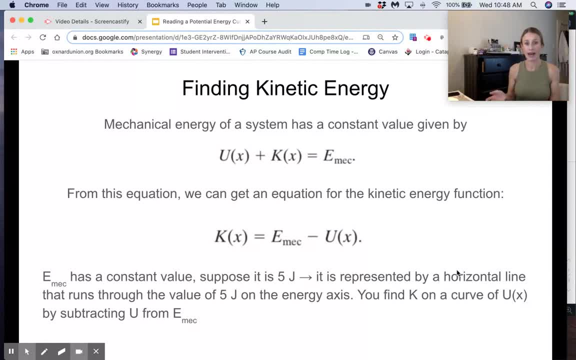 of energy. if you have no non-conservative forces, then we do have a constant value for mechanical energy. So suppose it's something like five joules. it's represented by a horizontal line drawn on the potential energy graph. So you'll see an example of this and they will give you. 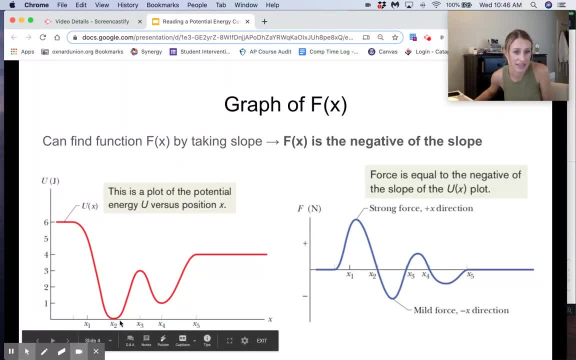 at x equals two. So we can see that Here we have a slope of zero here At x equals three. slope of zero here At x equals four. slope of zero here, And then after x equals five. slope of zero here. And then, as we go down here, 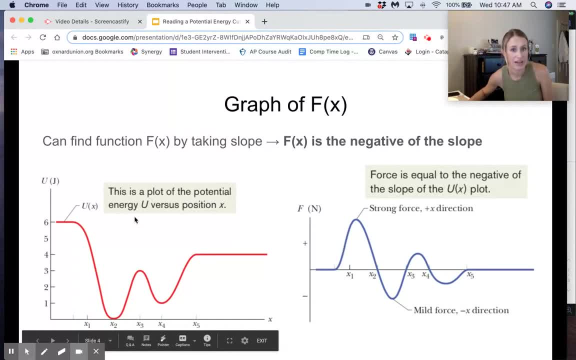 this is a negative slope. We have a positive force right here, And then here we can see that the slope is increasing, which means that the force is increasing. Here we have our largest positive force, And then it's going to decrease back to zero, which is why we're coming back down. 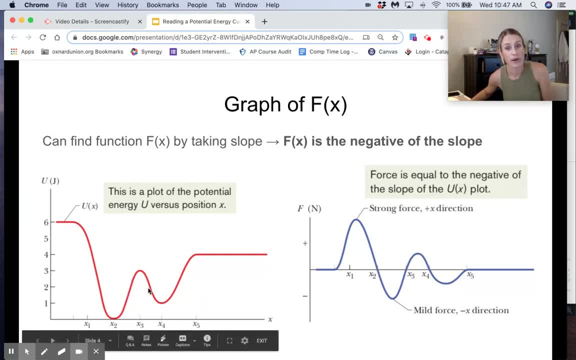 to zero here. Here our slope is lower in magnitude, so it doesn't get as high as here. but because it's a positive slope here, that means it's a negative force. and then here we have a slope that is negative, so we have a positive force here. and then here we have a positive slope, so we have 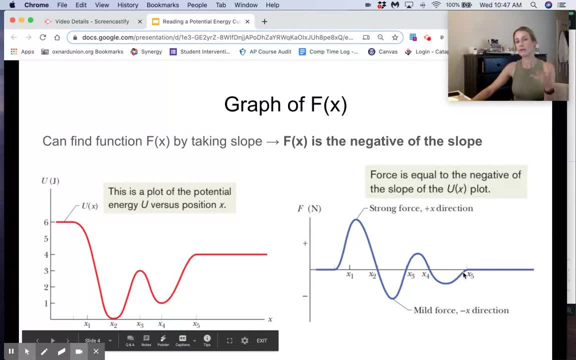 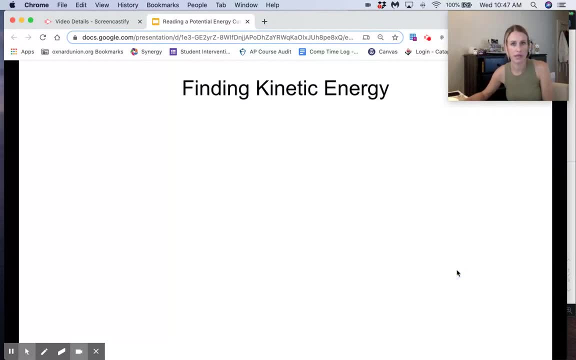 a negative force here. So you can kind of see how we could get a force graph from our potential energy graph. Now if we're trying to find kinetic energy from potential or a potential energy graph, we have to remember that mechanical energy of a system has a constant value that's given by 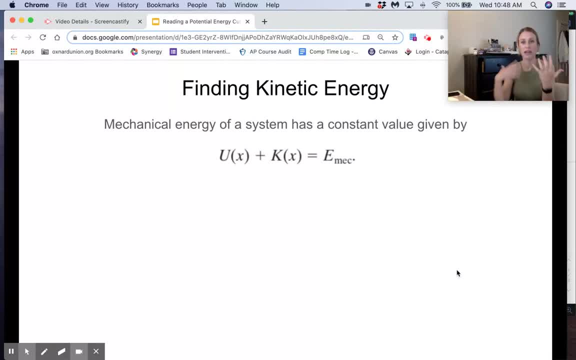 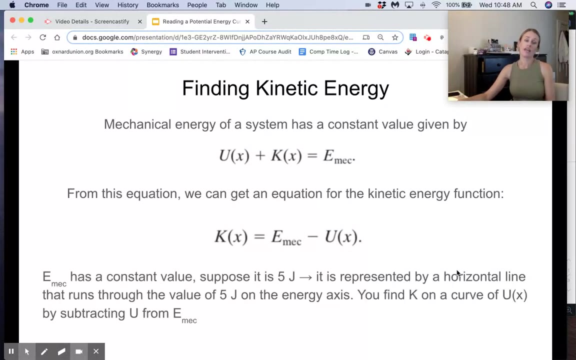 this right here: Mechanical energy is equal to a combination of potential energy plus kinetic energy. So from this equation we can get an equation for the kinetic energy function We get. kinetic energy is equal to total mechanical energy minus potential energy. So if we know that the total mechanical energy has a constant value, which we know from conservation, 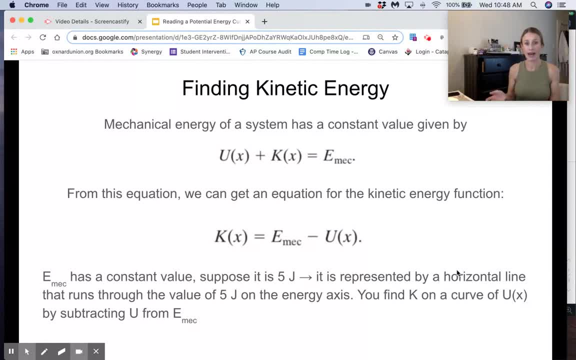 of energy. if you have no non-conservative forces, then we do have a constant value for mechanical energy. So suppose it's something like five joules. it's represented by a horizontal line drawn on the potential energy graph. So you'll see an example of this and they will give you. 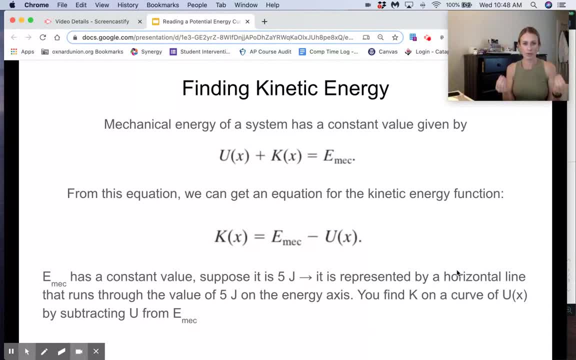 information in these problems to find the total mechanical energy. Once you find the total mechanical energy, then you draw a horizontal line at that point and then you can find kinetic energy on the curve by subtracting the potential energy from the total mechanical energy, So an? 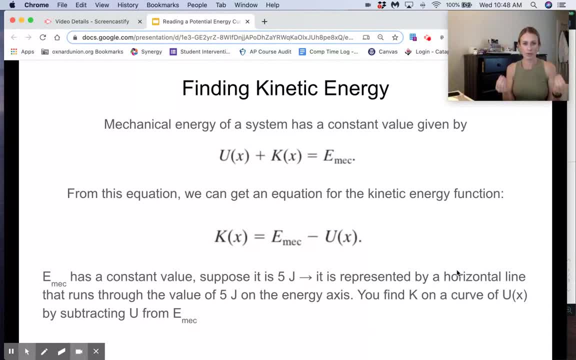 information in these problems to find the total mechanical energy. Once you find the total mechanical energy, then you draw a horizontal line at that point and then you can find kinetic energy on the curve by subtracting the potential energy from the total mechanical energy, So an? 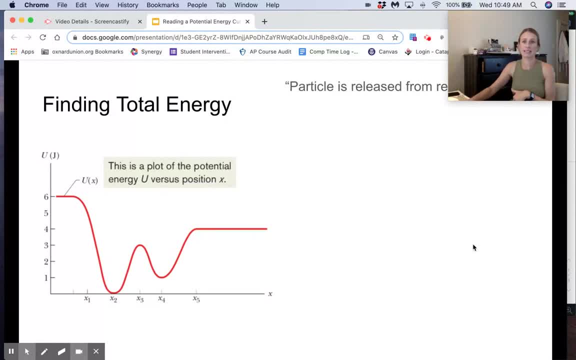 example of this here would be say: they would say something like: the particle is released from rest at x1 equals 2 meters. So what this tells us is that because our particle is released from rest at x1, rest means no kinetic energy. So what that means is that our particle is released from rest. 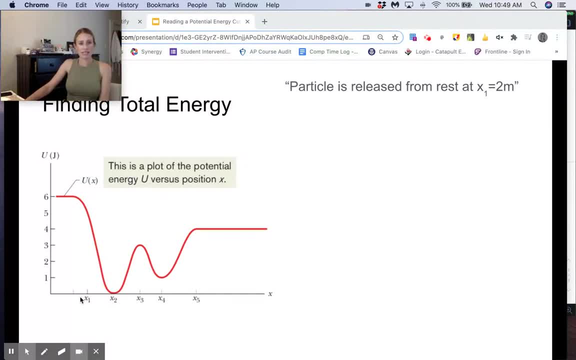 at x1.. So what that tells us is that at this position x1 right here, which is two meters, that means that we have all potential energy. So our potential energy is equal to our total mechanical energy. You would come up here, to this position x1, wherever we're at on this. 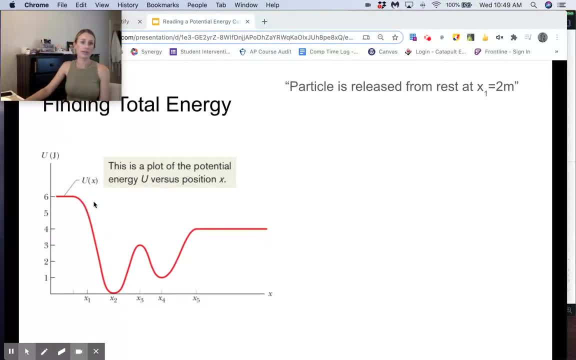 potential energy curve and you would draw a horizontal line at that point. So this means, like I said, that at two meters all of the particles, energies and potential energy would draw a horizontal line from the potential energy curve at that point to represent the total amount of energy. Another example would be: at x3 equals six meters, the particle has two joules of. 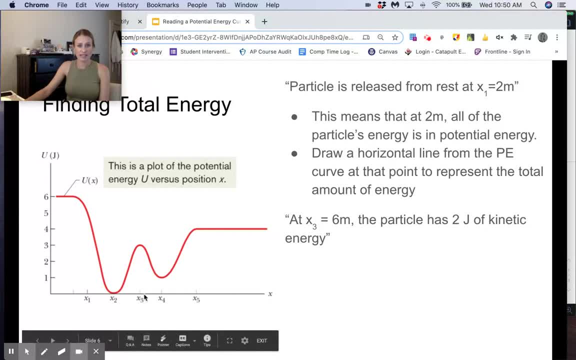 kinetic energy. So you would come here to this x3, which is six meters, and here I would see: okay, it looks like I have three joules of potential energy, and then it says the particle has two joules of kinetic energy. So I would then add two joules of kinetic energy to the potential energy. 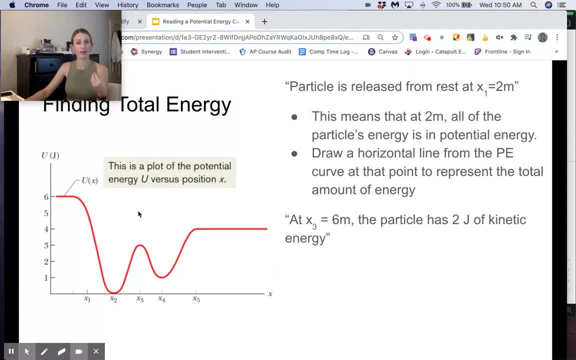 in order to get my total mechanical energy, because I know total mechanical energy is equal to kinetic energy plus potential energy. So that means that my total here would be three plus two, which is five, and then again I would draw a horizontal line at that five joule mark. 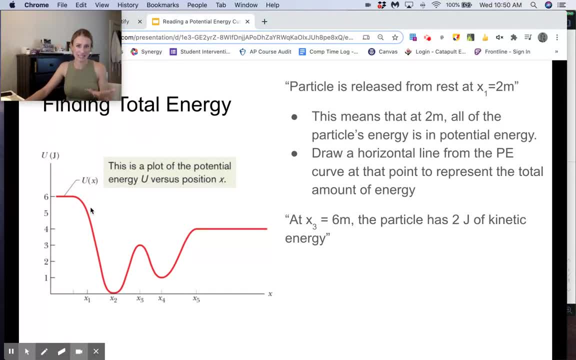 because that is my total mechanical energy and that is not going to be changing because of conservation of energy. So we would add this amount of energy to whatever potential energy the particle has at that point to get the total energy, and then you would draw a horizontal 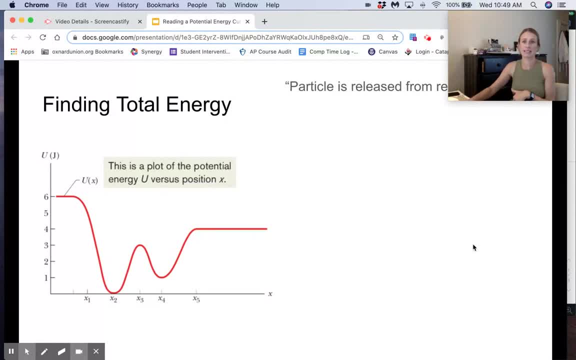 example of this here would be say: they would say something like: the particle is released from rest at x1 equals 2 meters. So what this tells us is that because our particle is released from rest at x1, rest means no kinetic energy. So what that means is that our particle is released from rest. 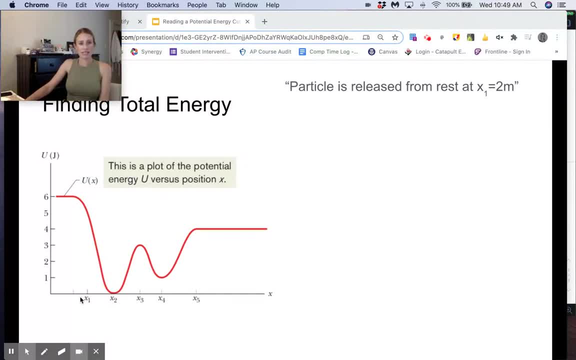 at x1.. So what that tells us is that at this position x1 right here, which is two meters, that means that we have all potential energy. So our potential energy is equal to our total mechanical energy. You would come up here, to this position x1, wherever we're at on this. 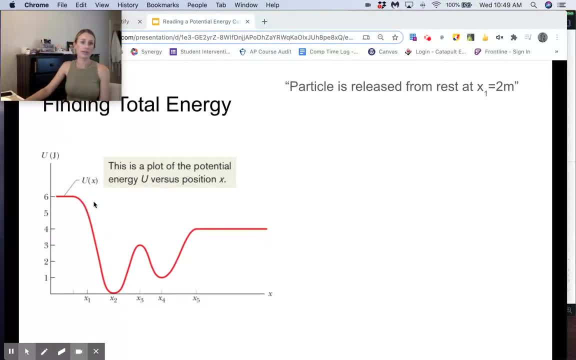 potential energy curve and you would draw a horizontal line at that point. So this means, like I said, that at two meters all of the particles, energies and potential energy would draw a horizontal line from the potential energy curve at that point to represent the total amount of energy. Another example would be: at x3 equals six meters, the particle has two joules of. 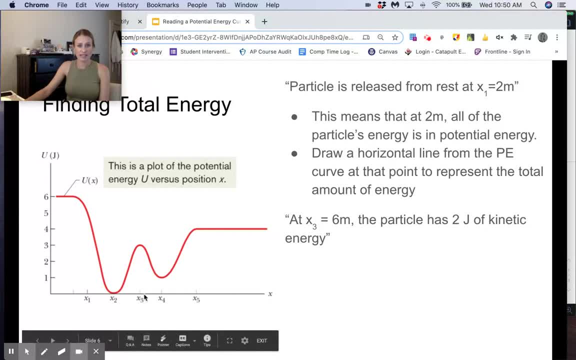 kinetic energy. So you would come here to this x3, which is six meters, and here I would see: okay, it looks like I have three joules of potential energy, and then it says the particle has two joules of kinetic energy. So I would then add two joules of kinetic energy to the potential energy. 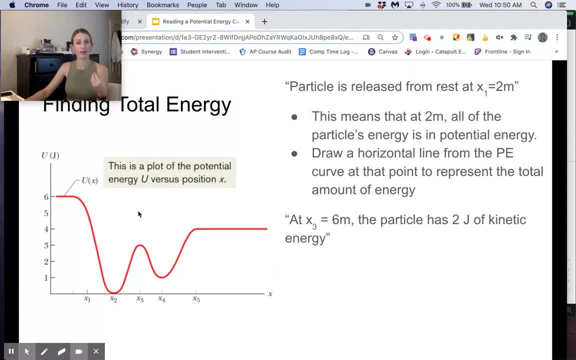 in order to get my total mechanical energy, because I know total mechanical energy is equal to kinetic energy plus potential energy. So that means that my total here would be three plus two, which is five, and then again I would draw a horizontal line at that five joule mark. 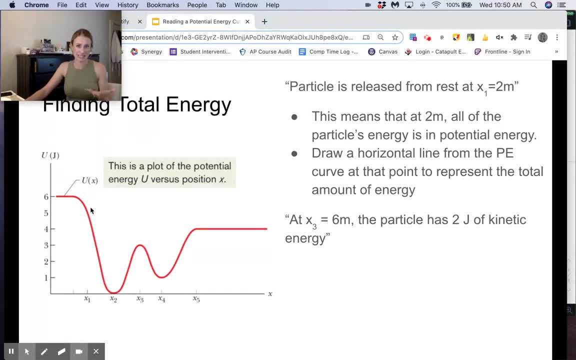 because that is my total mechanical energy and that is not going to be changing because of conservation of energy. So we would add this amount of energy to whatever potential energy the particle has at that point to get the total energy, and then you would draw a horizontal 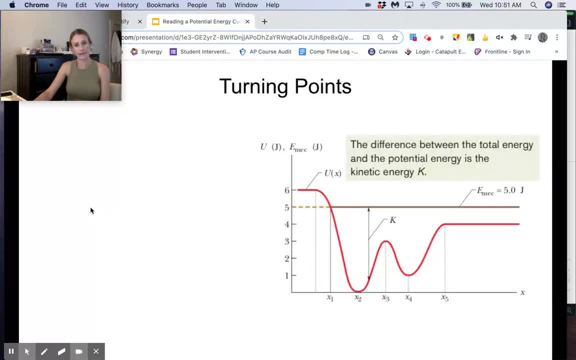 line at that point to represent the total energy. So once we do that, you can see here that with both of those examples I was given the total mechanical energy and I can see that I've drawn a horizontal line at that five joules because again, the total mechanical energy is not going to be changing. 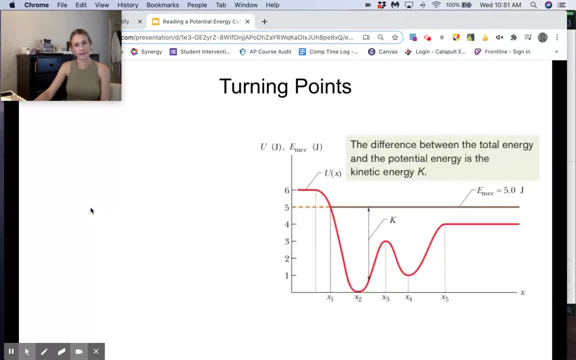 line at that point to represent the total energy. So once we do that, you can see here that with both of those examples I was given the total mechanical energy and I can see that I've drawn a horizontal line at that five joules, because again, the total mechanical energy is not going to be changing Now. 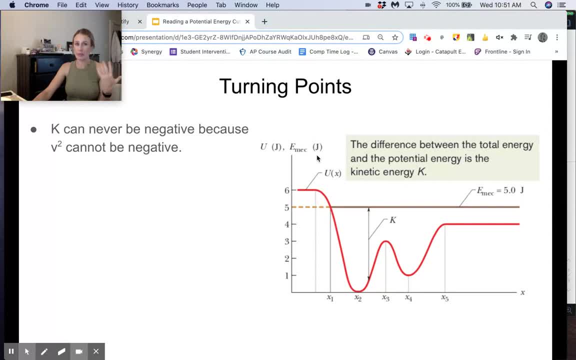 we're going to go ahead and change that. So a turning point is a place that we can't go beyond Now. the whole key here is that kinetic energy can never be negative because v squared can't be negative. So we know kinetic energy is equal to one half m v squared. Mass isn't negative Velocity. 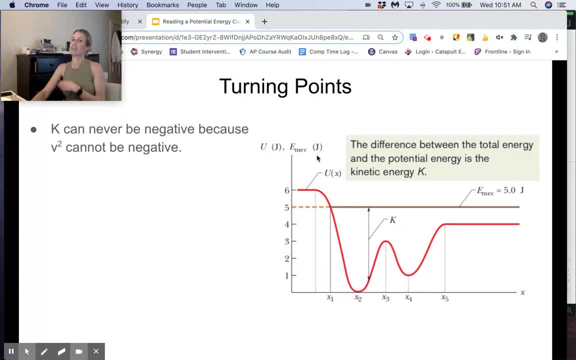 could be negative. but a negative times a negative can never be negative. So because of that, kinetic energy itself can't be negative. So because of this, the point where that mechanical energy line meets the potential energy curve, we call this a turning point, which is like this point: 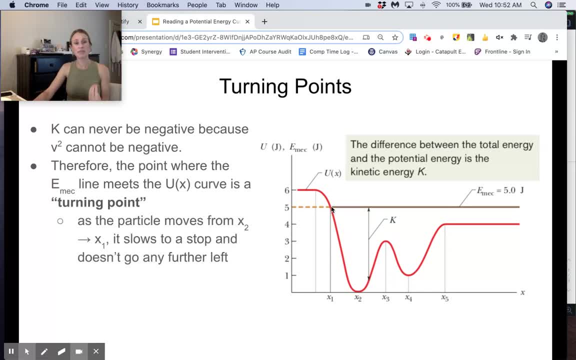 right here, Okay. So what happens here is, as the particle moves from, say, our position X2 to our position X1, which is where our turning point is located- it slows to a stop because we can see that the difference from this potential energy to the mechanical energy that's going to be our 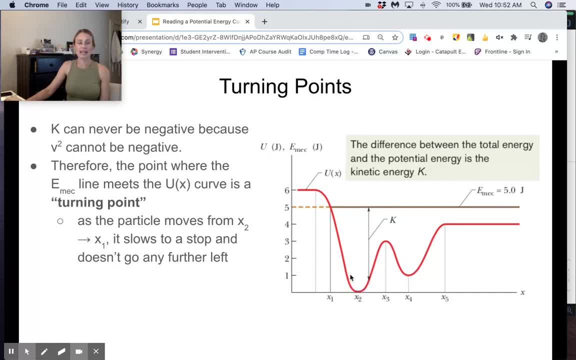 kinetic energy. So we can see here that, sorry, kinetic energy is decreasing, decreasing, decreasing, and then that means it's slowing to a stop here and it can't move any farther left. because again it can't be negative. We can't go above this total mechanical energy line. 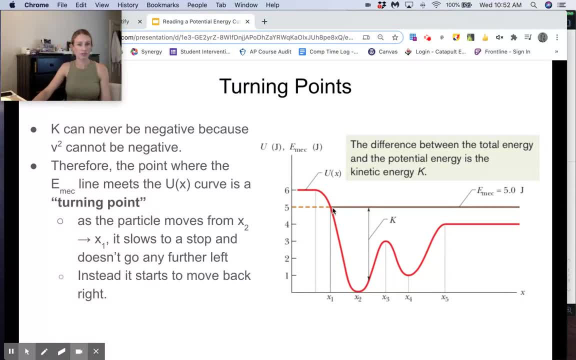 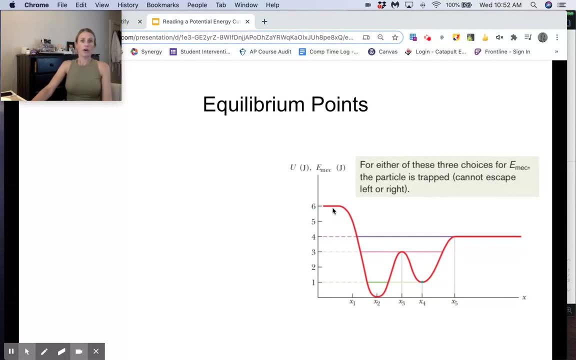 So because of that, instead it starts to move back to the right. So it turns around- which is why it's called a turning point- and it moves back to the right. So we also have these things called equilibrium points. So in these examples we have different total mechanical energy. So I know that. 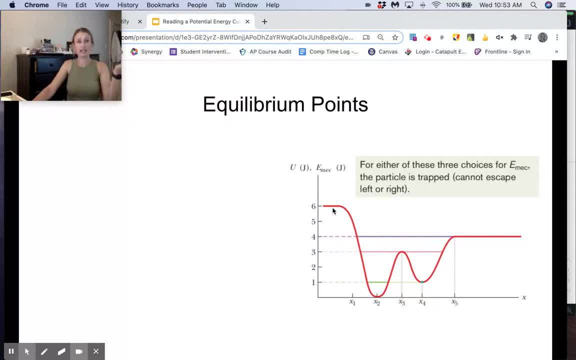 I've been talking about a total mechanical energy of five joules in our last examples, but here it's when we're changing the total mechanical energy amount that we get these what we call equilibrium points. So you'll see what I mean when we start explaining. So if if say my total, 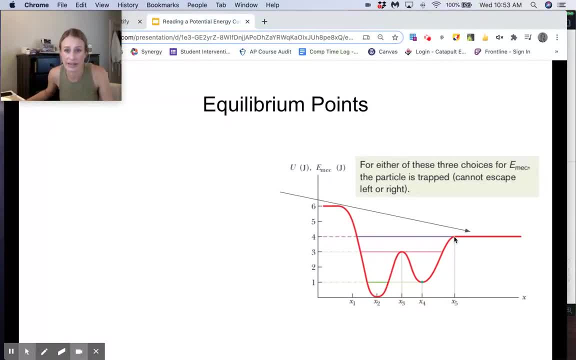 mechanical energy is four joules, so I draw a line Here at four joules, if I get to this plateau right here. this is called a neutral equilibrium. All right, neutral equilibrium. So we have a system's mechanical energy is equal to its. 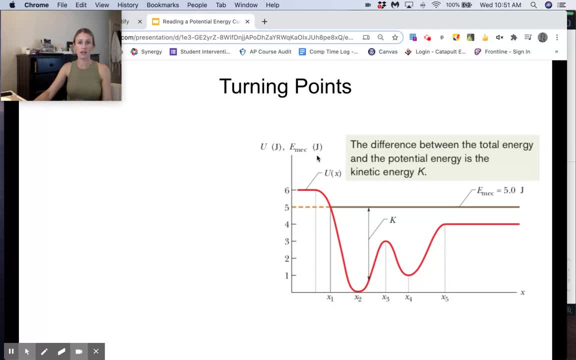 Now, because of this, we get these things called turning points. So a turning point is a place that we can't go beyond. Now the whole key here is that kinetic energy can never be negative, because v squared can't be negative. So we know kinetic energy is. 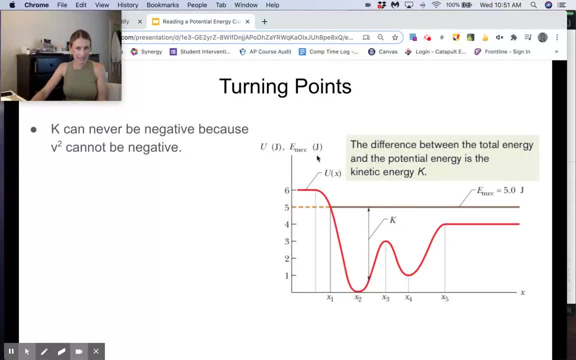 equal to one half m v squared Mass isn't negative. Velocity could be negative, but a negative times a negative can never be negative. So because of that, kinetic energy itself can't be negative. So because of this, the point where that mechanical energy line meets the potential energy curve, we call this a turning point, which is like this: 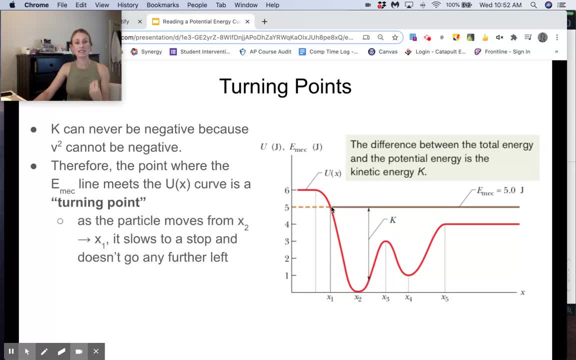 point right here. Okay, so what happens here is, as the particle moves from, say, our position x2 to our position x1, which is where our turning point is located, it slows to a stop because we can see that the difference from this potential energy to the mechanical energy that's going to 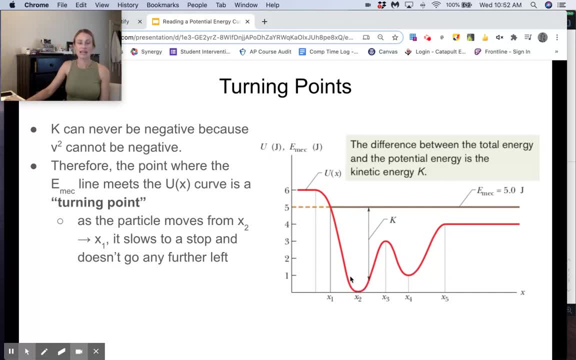 be our kinetic energy. So we can see here that sorry, kinetic energy is decreasing and then that means it's slowing to a stop here and it can't move any farther left because again it can't be negative. We can't go above this total mechanical energy line. So because of that, 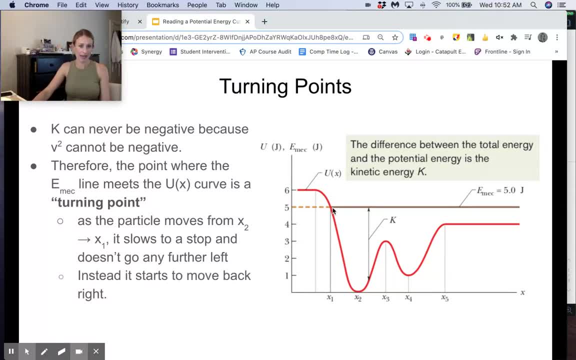 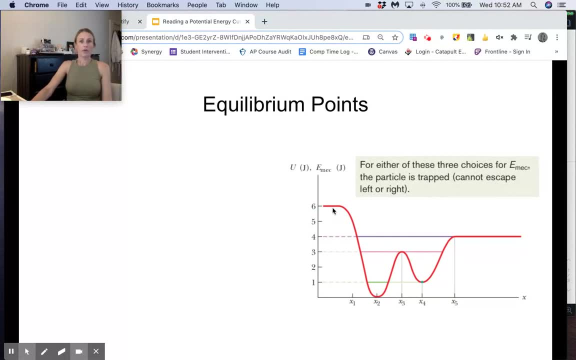 instead it starts to move back to the right. So it turns around- which is why it's called a turning point- and it moves back to the right. So we also have these things called equilibrium points. So in these examples we have these two points. 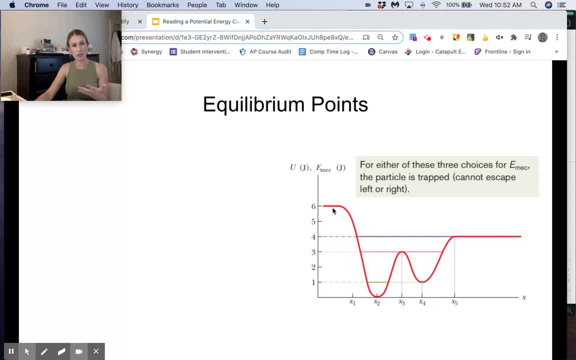 So I know that I've been talking about a total mechanical energy of five joules in our last examples, but here it's when we're changing the total mechanical energy amount that we get these what we call equilibrium points. So you'll see what I mean when we start explaining. So if 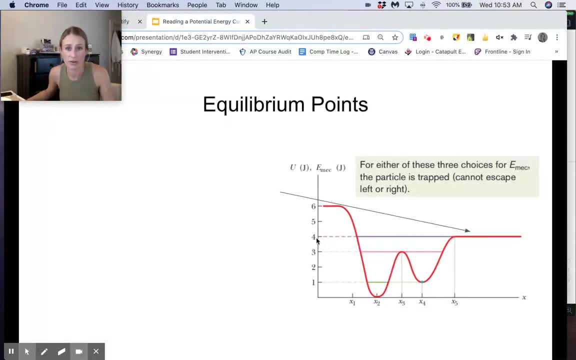 if, say, my total mechanical energy is four joules, so I draw a line here at four joules if I get to this plateau right here, this plateau here. this is called a neutral equilibrium. All right, neutral equilibrium. So we have a system's. 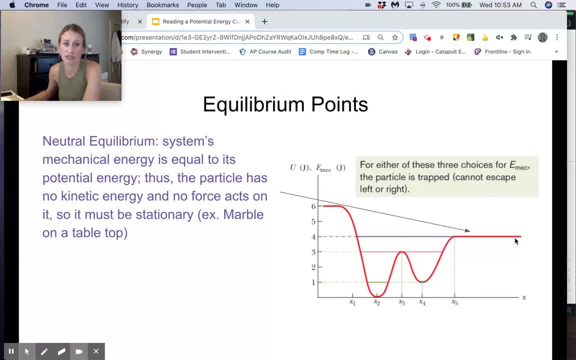 mechanical energy is equal to its potential energy in a neutral equilibrium. So we can see here: our total mechanical energy is that four joules. and then at this plateau right here beyond x5, we can see that that's what our potential energy is equal to. So all of the energy is in potential. 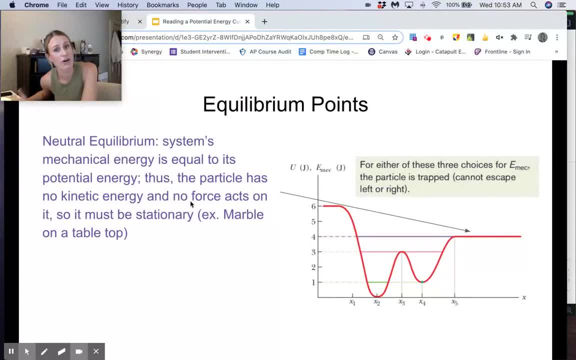 energy. Now here, the particle has no kinetic energy and no force acts on it, because we can see that the slope here is zero, so that particle must be stationary. This is called a neutral equilibrium. An example of this would be like a marble on a tabletop right: There's no forces. 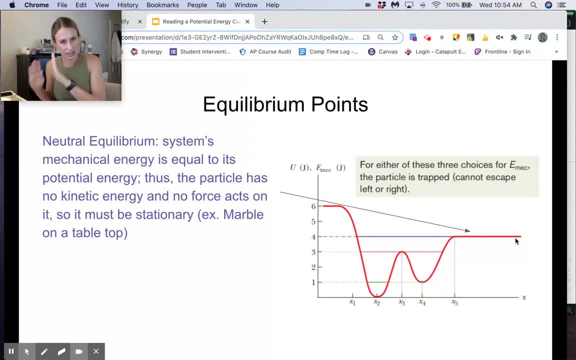 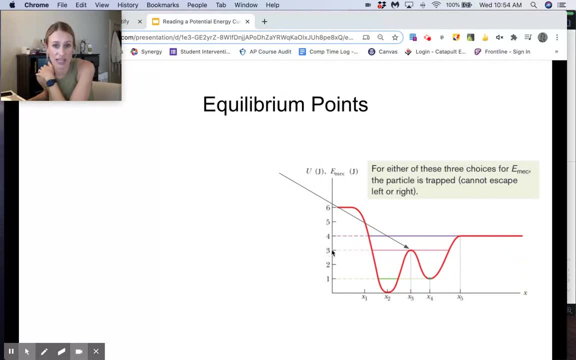 acting on the marble to the left or to the right, so that marble is in neutral equilibrium. Now, instead, if we have, say, our total mechanical energy of three joules and we draw again our horizontal line right here, this point right here is called an unstable equilibrium. 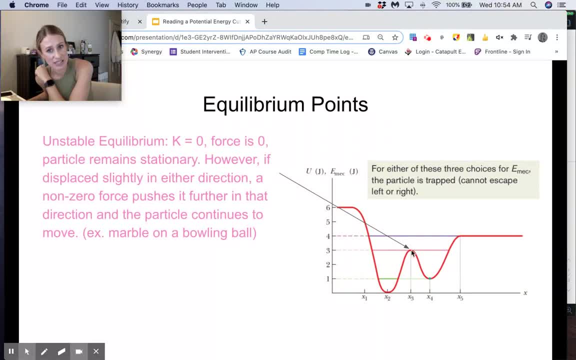 Now, here again, our kinetic energy is equal to zero, because we can see that total mechanical energy is three joules and also our potential energy is also three joules. So all of the energy is in potential energy. But we can also see that although our force is zero, it's very precarious. 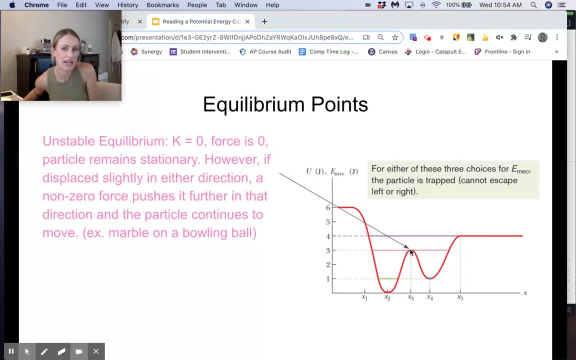 here right, Like if we move a little bit to the left or a little bit to the right, we now have a non-zero force which is going to then force it in one or the other direction. So we have a kinetic energy of zero here. force is zero because the slope of this curve at this. 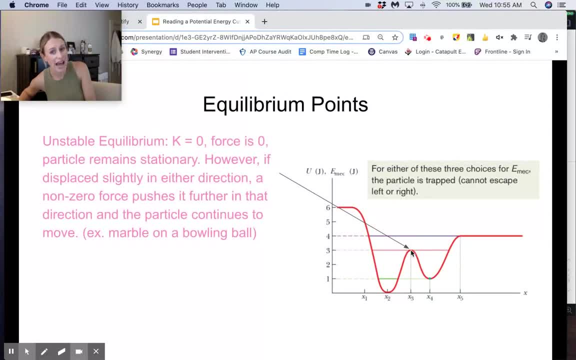 point x3 is also zero. However, if it's displaced slightly in either direction, a non-zero force is then going to push it farther in that direction, and then the particle will continue to move. So if we have something like a marble on a bowling ball right, It could balance there. 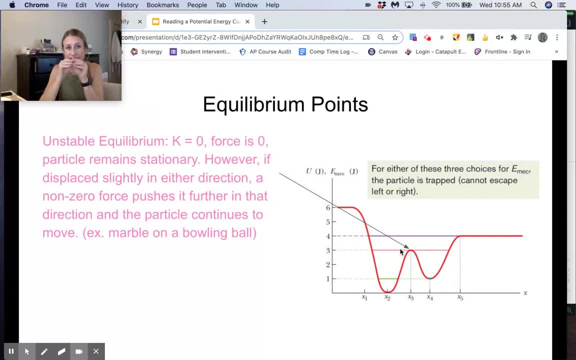 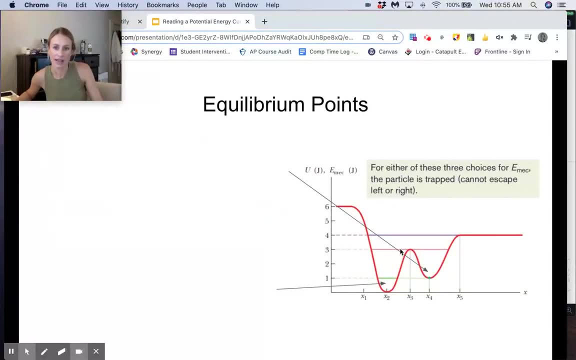 but it's very precarious. So this is an unstable equilibrium. So we have a non-zero force here, but we have a non-zero force here. So this is an unstable equilibrium point. Okay, and now for our last couple examples. here we have a total mechanical energy of one joule. 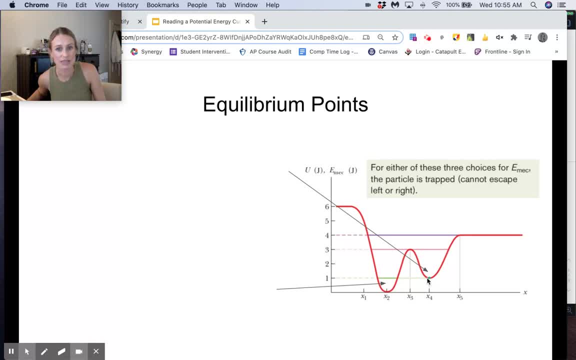 So now we're drawing our horizontal line at this point right here and we have two different equilibrium points. So our first one is, at this point right here, x4.. So this is called a stable equilibrium. Now, here in a stable equilibrium, our particle is stuck, all right, It can't move. 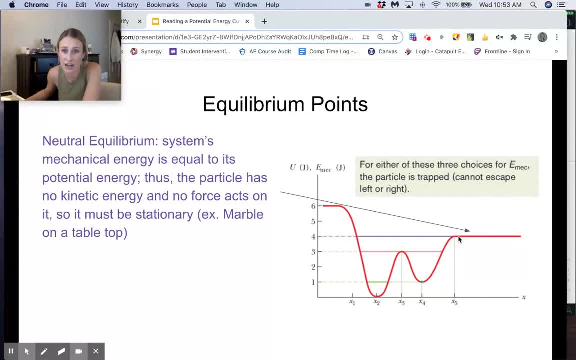 potential energy in a neutral equilibrium. So we can see here: our total mechanical energy is that four joules. And then at this plateau right here, beyond X five, we can see that that's what our potential energy is equal to. So all of the energy is in potential energy. 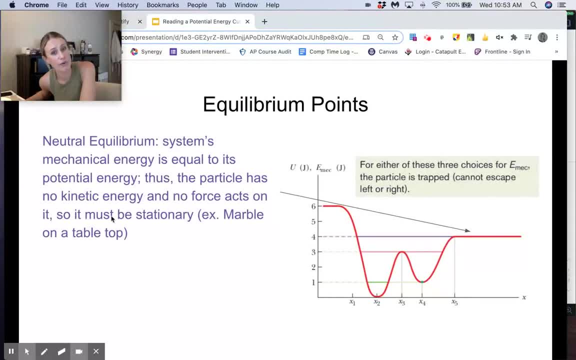 Now here, the particle has no kinetic energy and no force acts on it, because we can see that the slope here is zero, So that particle must be stationary. This is called a neutral equilibrium. An example of this would be like a marble on a tabletop right. 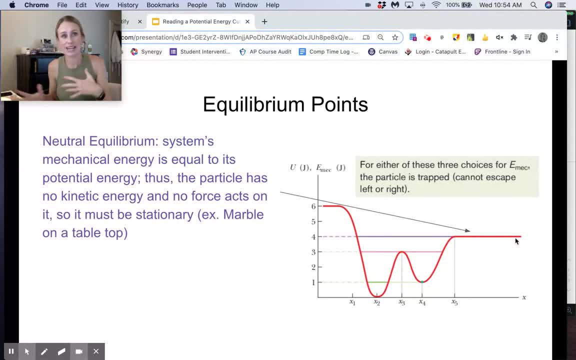 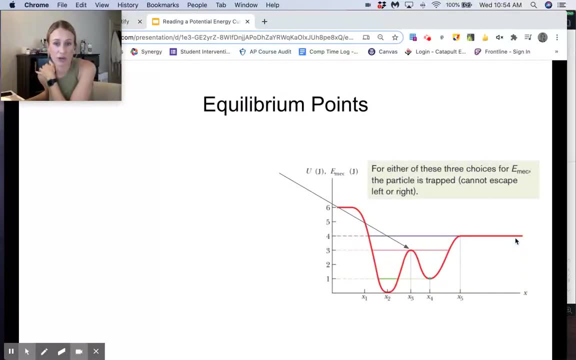 There's no forces acting on the marble to the left or to the right, So that marble is in neutral equilibrium. Now, instead, if we have, say, our total mechanical energy of three joules and we draw again our horizontal line right here, this point right here is called an unstable equilibrium. 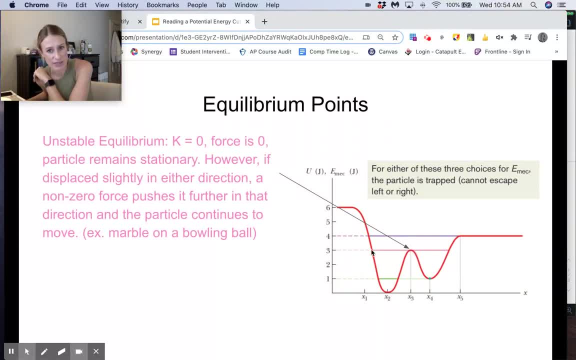 Now, here again, our kinetic energy is equal to zero, because we can see that total mechanical energy is three joules And also our potential energy is also three joules. So all of the energy is in potential energy. But we can also see that although our force is zero, it's very precarious. 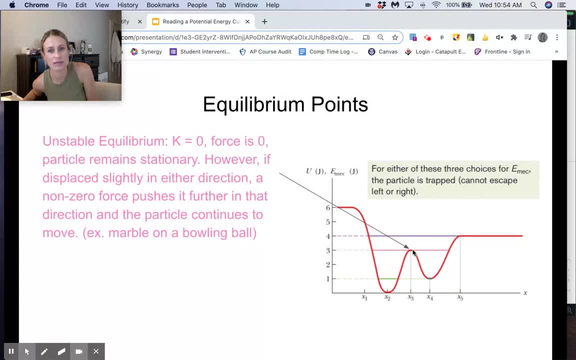 here right, Like if we move a little bit to the left, we can see that our force is zero, And or slightly further to the left or a little bit to the right, we now have a nonzero force which is going to then force it in one of those directions And therefore we will then start moving. 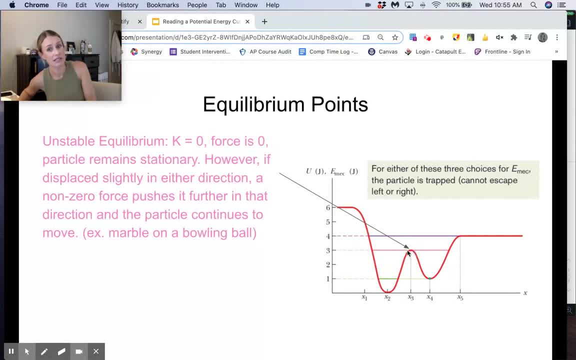 So we have a kinetic energy of zero here. The force is zero because the slope of this curve, at this point x3, is also zero. However, if it's displaced slightly in either direction, a nonzero force is then going to push it farther in that direction, and then the particle will continue to move. 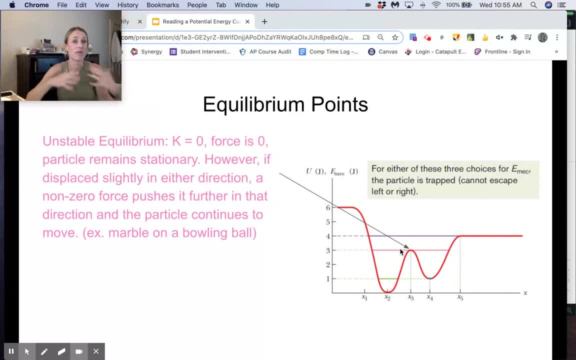 And then the particle will continue to move. So if we have something in between here and thing along the trying to this path, something like a marble on a bowling ball, right, It could balance there, but it's very precarious. So this is an unstable equilibrium point. Okay, and now for our last couple examples. here we have: 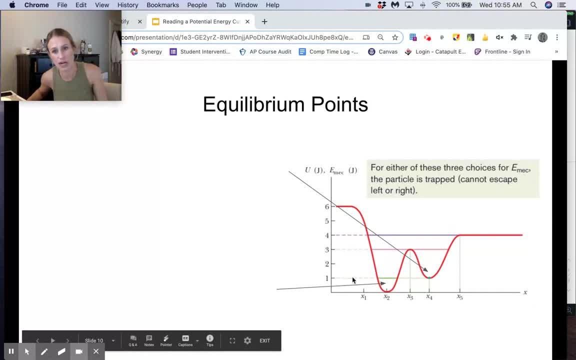 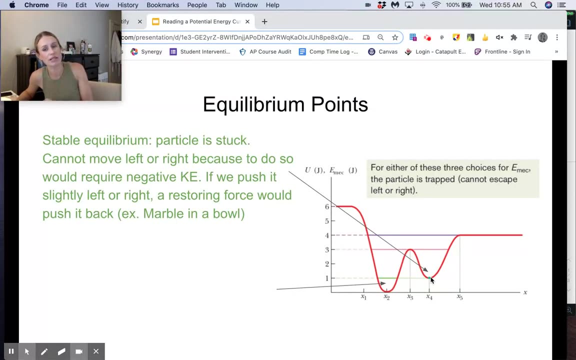 a total mechanical energy of one joule. So now we're drawing our horizontal line at this point right here, and we have two different equilibrium points. So our first one is, at this point right here, x4.. So this is called a stable equilibrium. Now, here, in a stable equilibrium, our particle is: